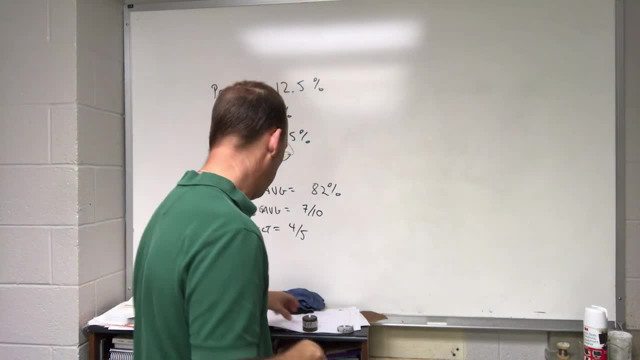 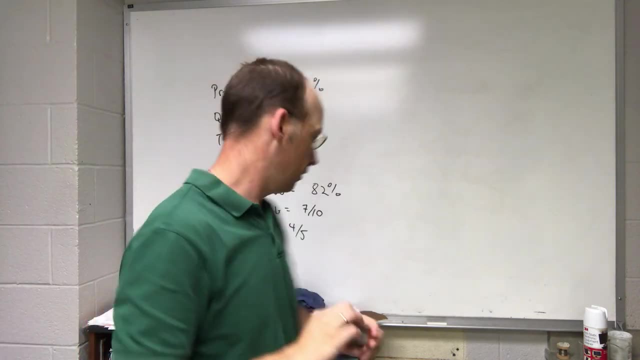 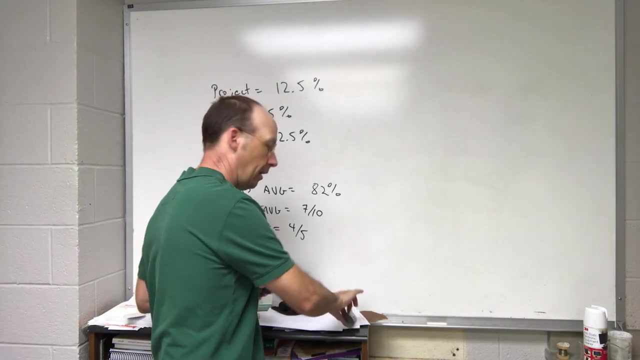 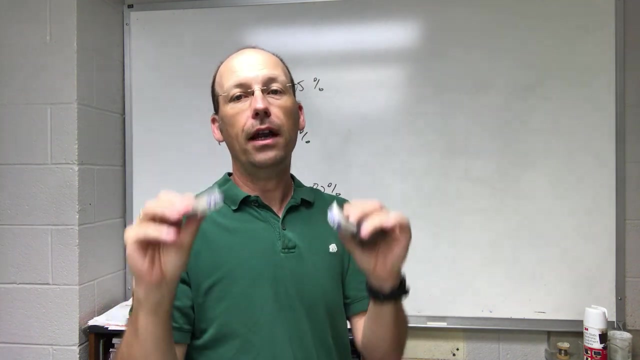 Okay. so here's the situation. I made up a situation. It's not real. You have three things in your course. You have tests- It's this math right here, See, it's worth a lot. You have quizzes- It's not as much, but it's still pretty significant- And then you have a project which is just a little bit. So these all count for different amounts. Finding the average grade is like finding the center mass for these three things. 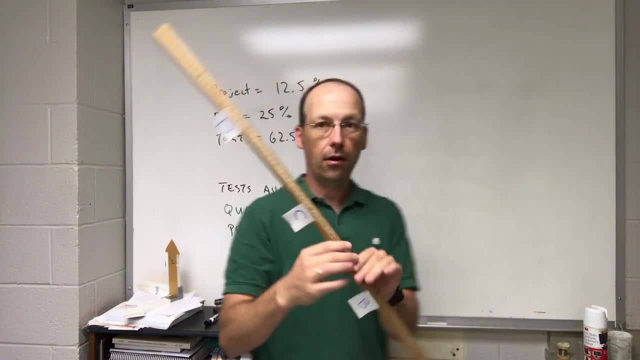 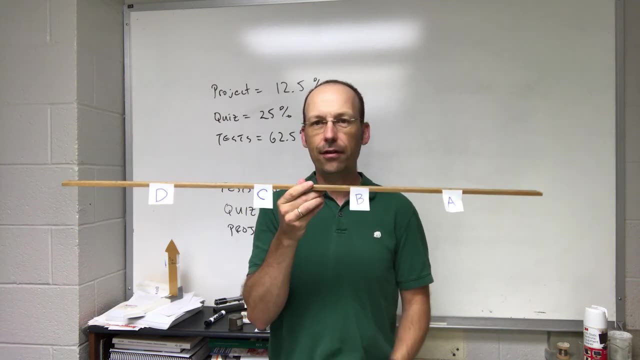 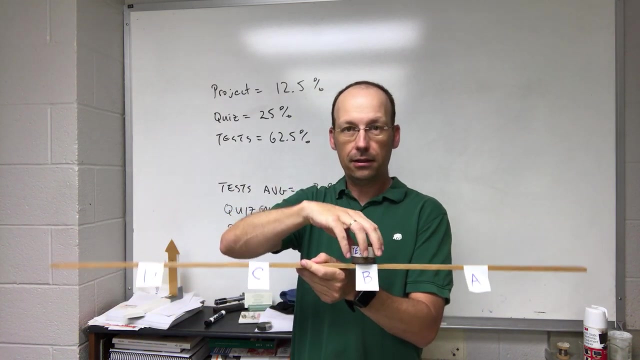 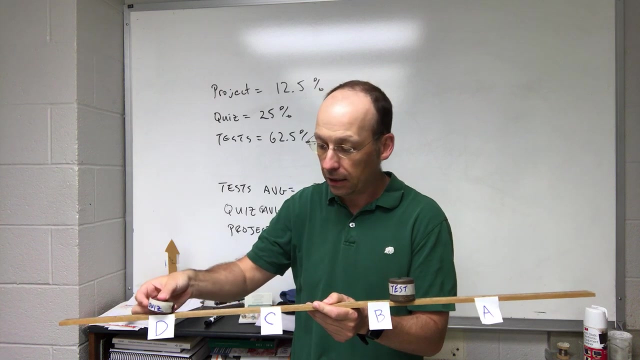 So let me show you, Let me do a little demo here. Okay, so here is A, B, C, D, evenly spaced out. F's not on there because you don't want to get an F, Okay, so let's put these on here. So let's say I do, I get a B on the test. Or let's say it's a little bit higher than a B And then I do really poorly on the quiz. I get a D, Okay, and then I get, I do a middle C. 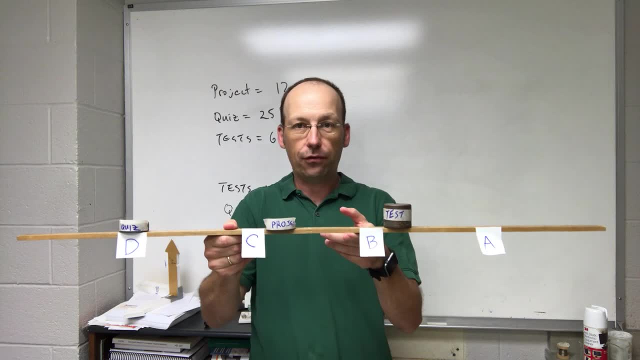 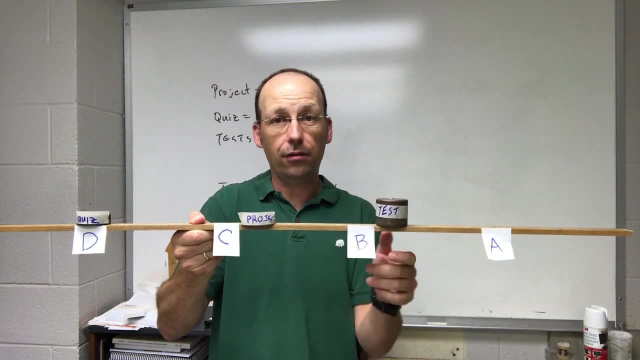 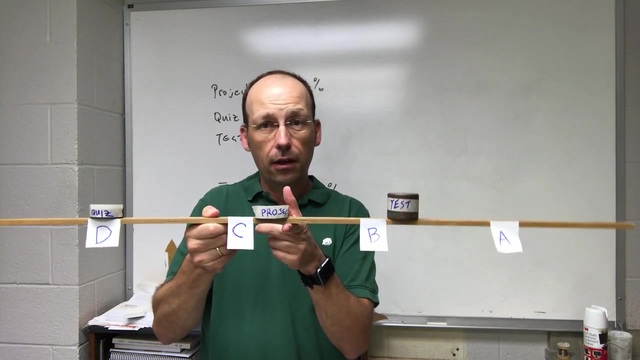 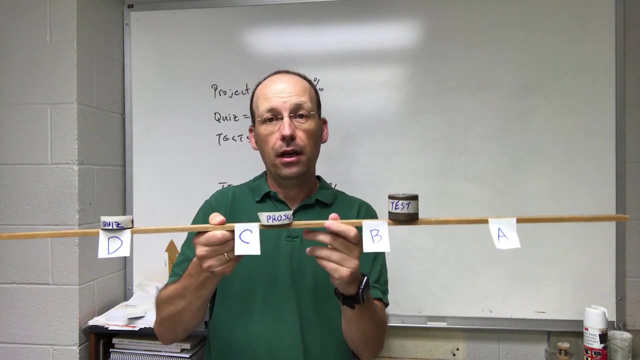 Right there. So then, where is the center of mass for this whole thing? Is it a, B Or is it the average of these strings? No, it's not. So it depends on both the mass and the location of these things. So this is going to be closer to this one, because it's going to be somewhere around here. Because this has more weight, It's weighted higher than the other thing, So it matters more. When you calculate the center mass, it matters more, And we're going to do a problem that's essentially the same thing as calculating the center mass. 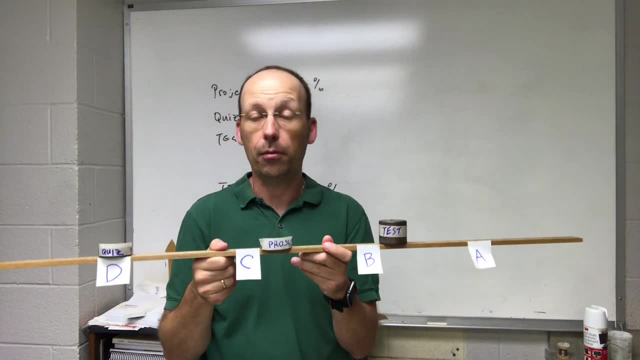 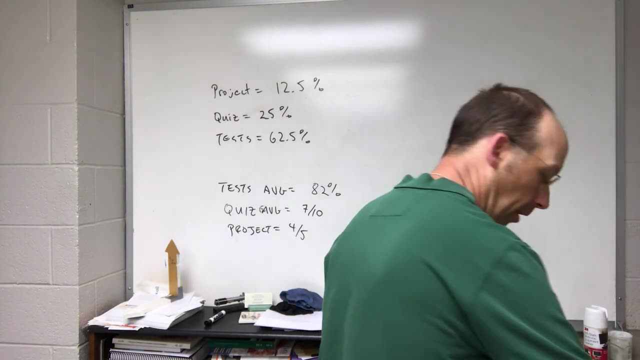 For this system, And that's what we're going to do right now. Okay, I'm going to use some numbers. I made up a fake course with fake grades And I didn't even drop my courses, my grades, They fell off the thing. 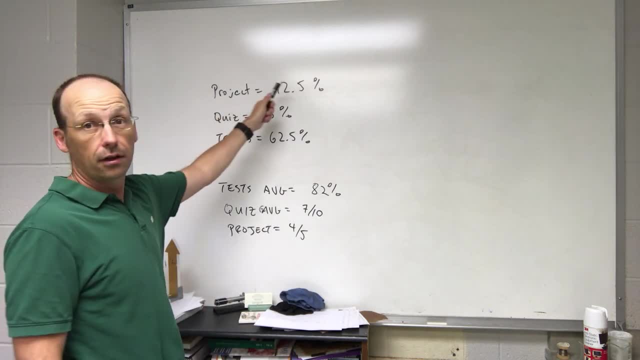 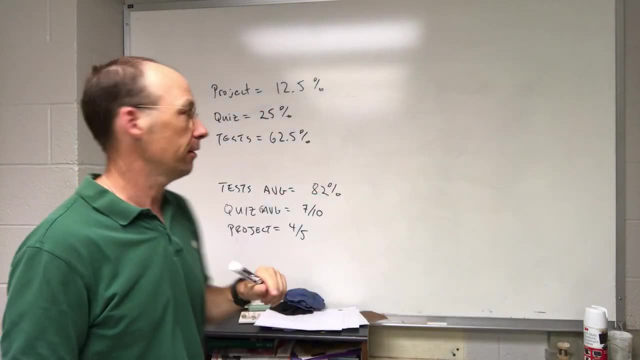 Okay, so here's my course. It has a project worth 12.5%, And I got that number because that's 100 grams out of 800.. That was the same weight as the thing. And then I have the quiz worth 25%. It was 200 grams. 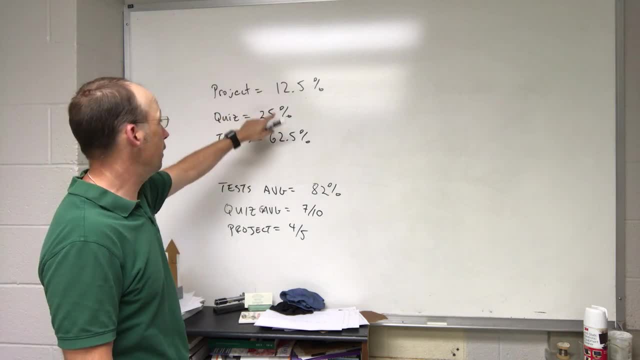 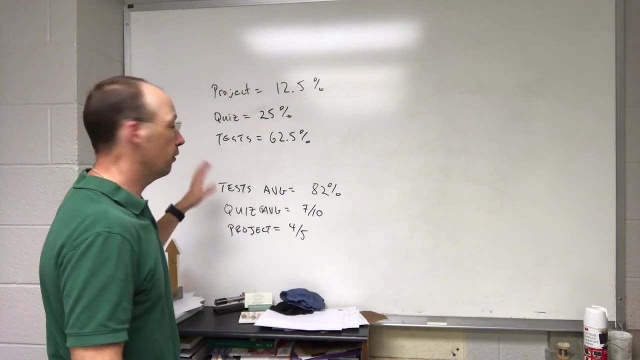 And then the test is 62.5% And if you add these all up you get 100%. The course should add up to 100%, Unless you're not complete. And then here's what you did: You have your test average is an 82%. 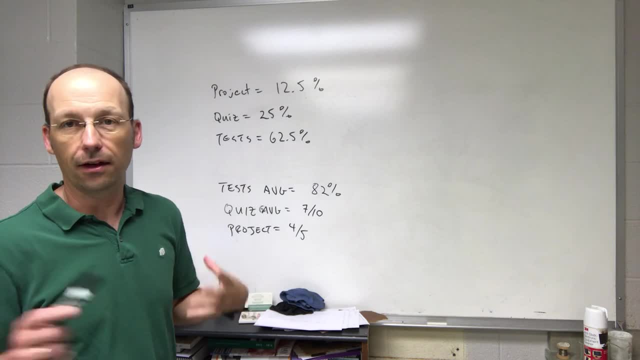 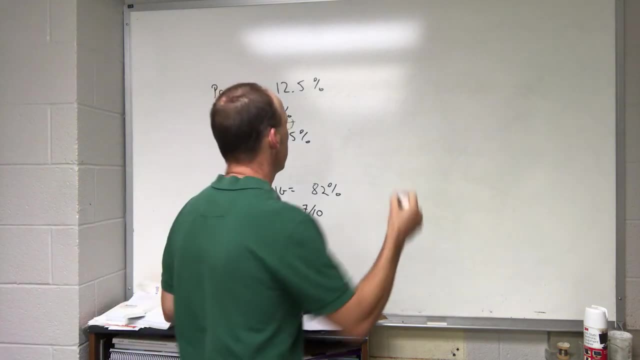 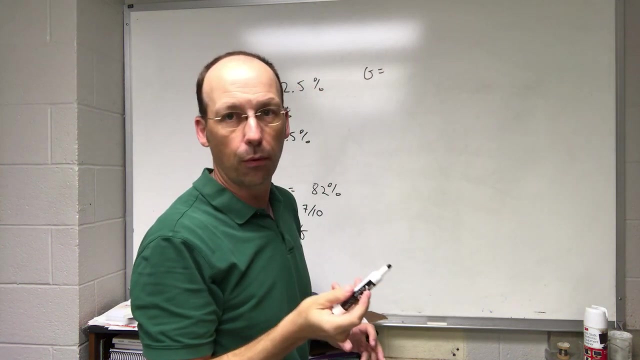 Your quiz is 7 out of 10.. I threw that in there Just to be fun. And then your project is 4 out of 5.. So the grade is calculated as following Grade is going to be equal to. I'll write this out in a simple way. 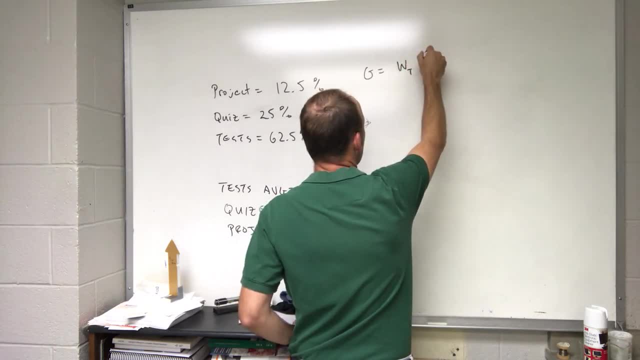 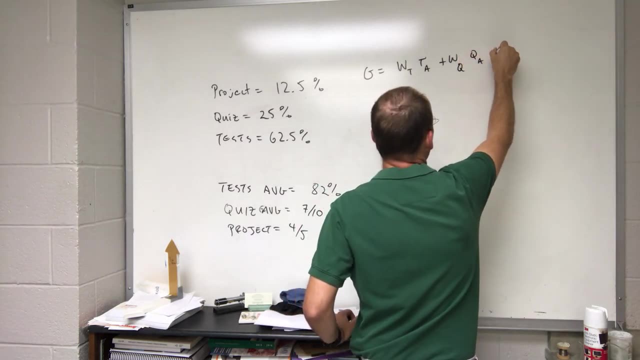 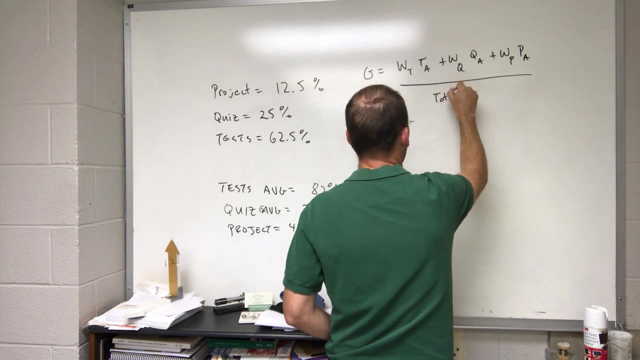 It's going to be the weight of the test times, your test average plus the weight of the quiz times, the quiz average plus the weight of the project times, the project average divided by total weight. Now, in this case, my total weight is 1.. 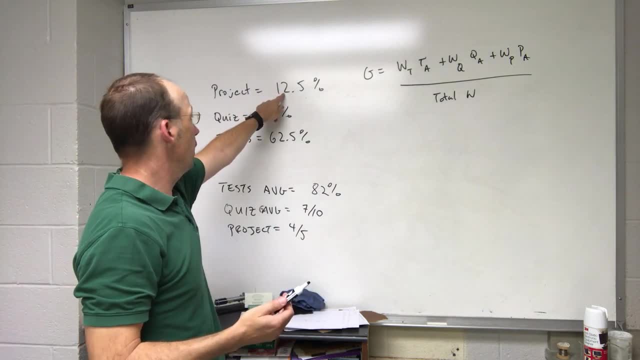 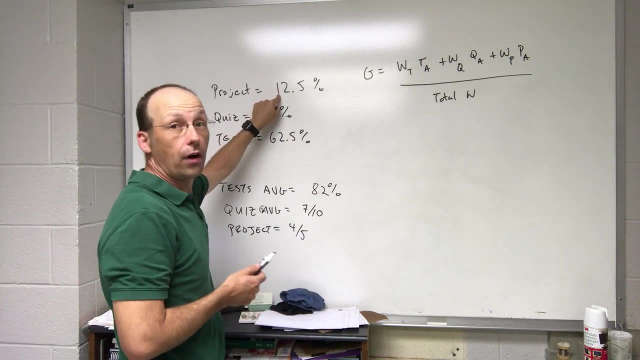 That's what I want, right? 1. Each, Each These are. If I turn these 2% to decimals and add them up, I get 1.. So that's what I'm going to do. I'm going to use my weight as 0.125 and weight of 0.25 and weight of 0.625.. 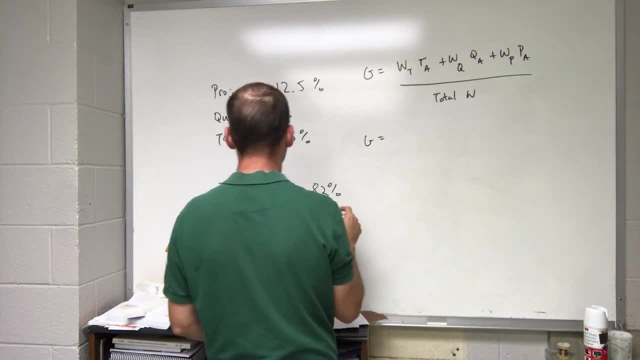 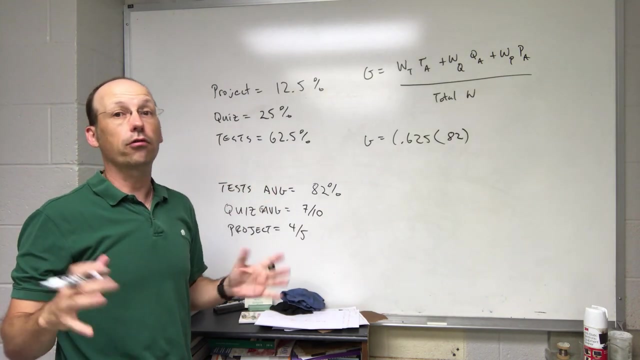 So let's calculate the grade. Okay, so my test is worth 62.5%, So I'm going to say 0.625 times the test average of 82%. Now I'm going to leave that, as I'm going to leave all my grades as a fraction of 100.. 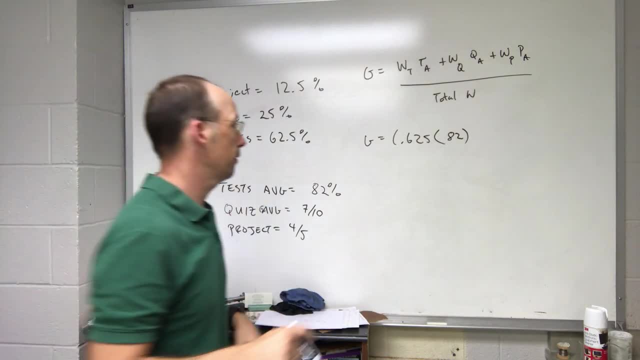 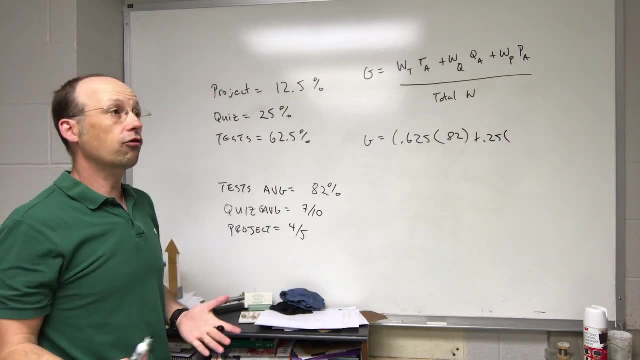 Because you want your. You want your grade at the end to be out of 100., But you could do it either way you want. Plus, the weight of the quiz is 0.25.. Now what is my grade out of 100 if I have 7 out of 10?? 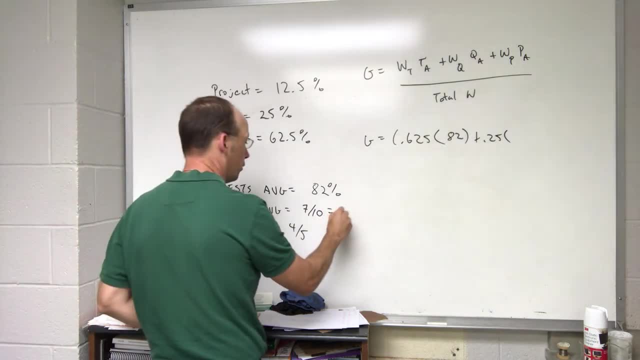 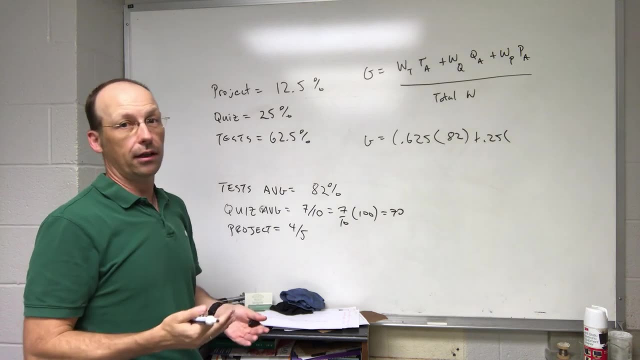 Well, it's going to be the percent, So it's going to be equal to 7. divided by 10 times 100 equals 70.. So that's my percent, correct in the grade. I could write that out up there, but I'm just going to put 70.. 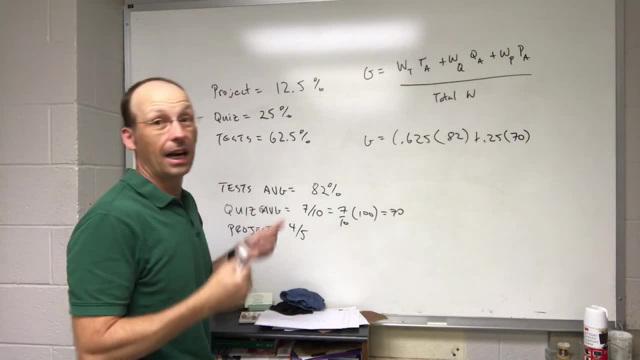 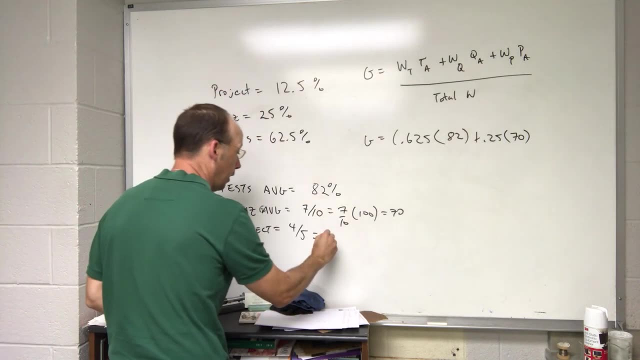 Just to save space, But that's how you. You've got to get that into the same. These have to be the same format, And then down here I need to do the same thing. This is going to be 4 out of 5 times 100.. 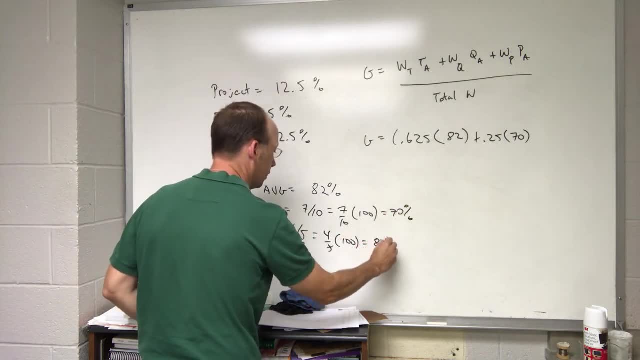 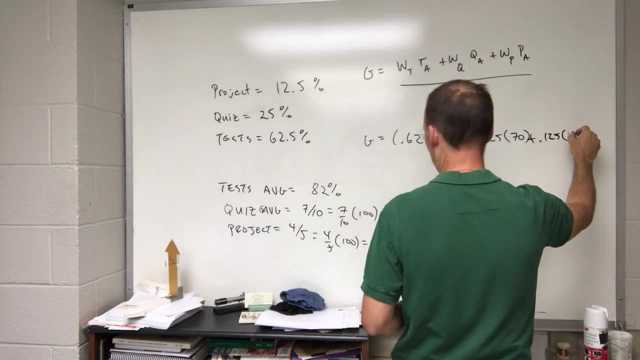 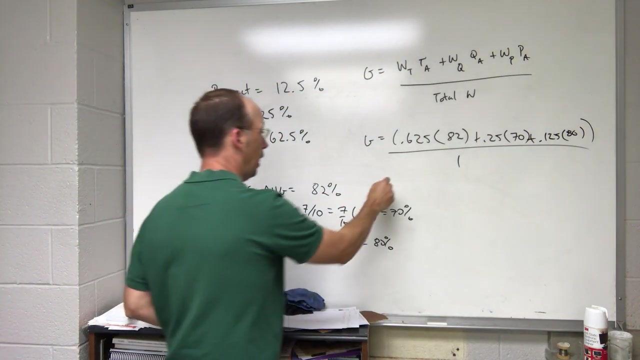 That's percent Equals 80%. So I'm going to put plus 0.125 times 80. And then all of that divided by 1., Because It all adds up to 1.. And if I do that, and I put that in my calculator, which I already did- 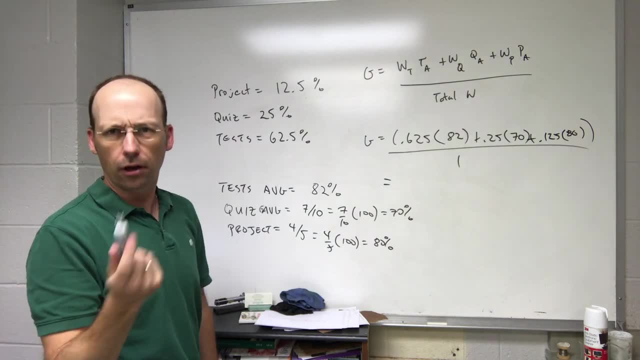 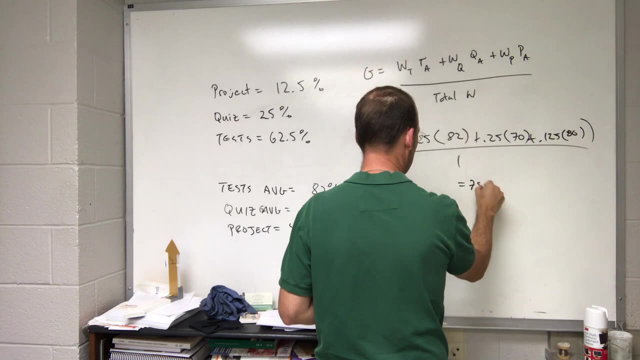 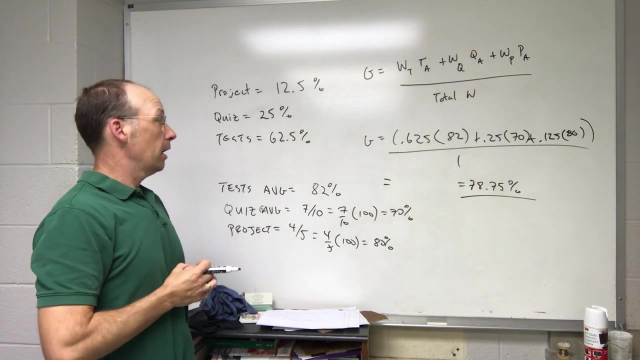 because I wanted to save time. Because now I'm wasting time by talking about how I save time. Okay, so then I get 78.75.. So that's my grade in the course. Okay, Now let's do another situation that does happen. 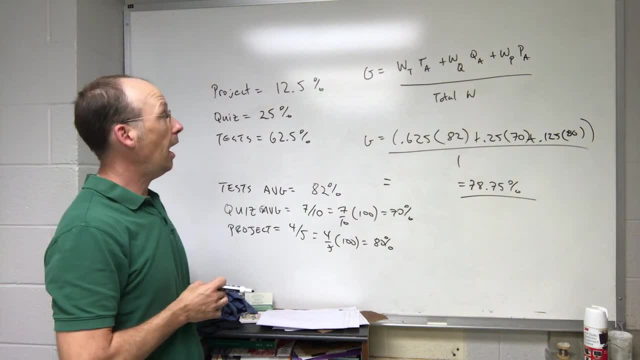 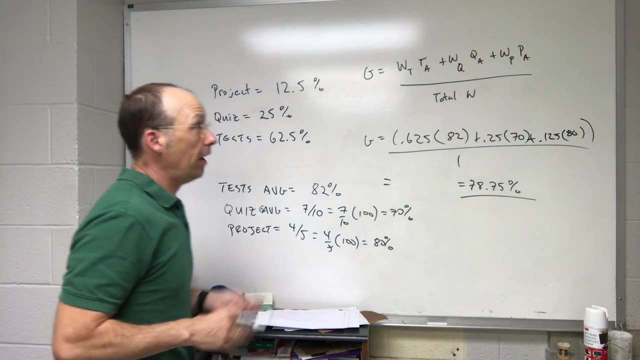 Suppose you're not finished with the course and you want to calculate your grade. I haven't done the project. I've only completed the test and the quiz. What's my grade going to be? Well, if I haven't done the project, I can't average the project in. 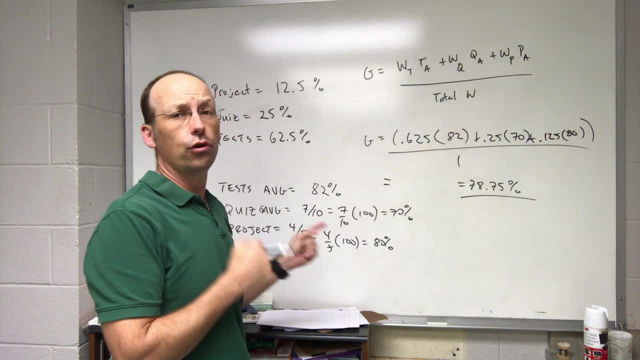 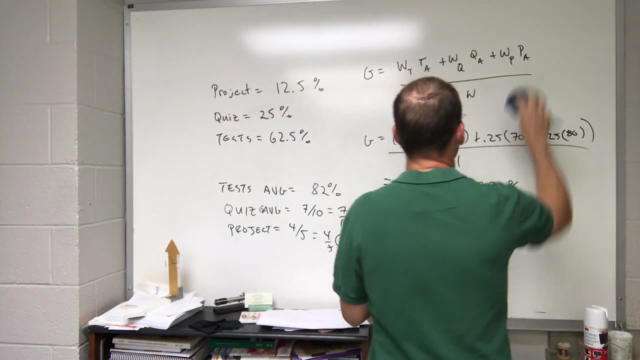 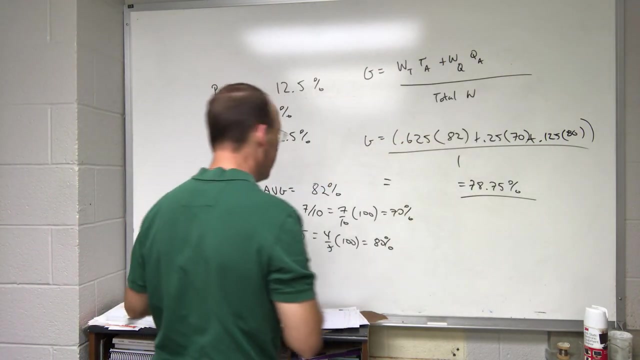 You could, of course, guess and say: I think I'm going to get this grade and put it in there, But if you're wrong, you're wrong. Okay, But let's just delete that. So what changes is now? my total weight is not 1.. 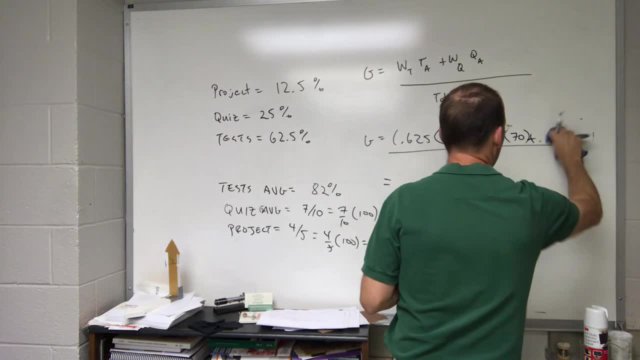 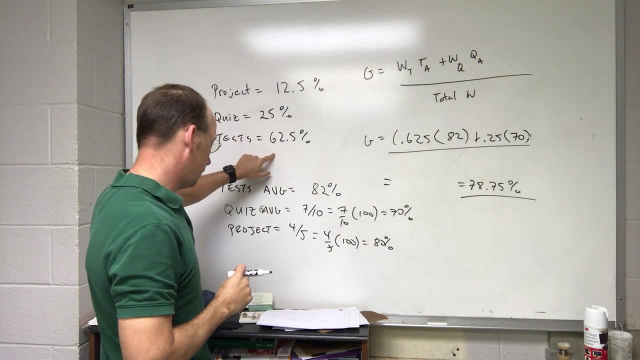 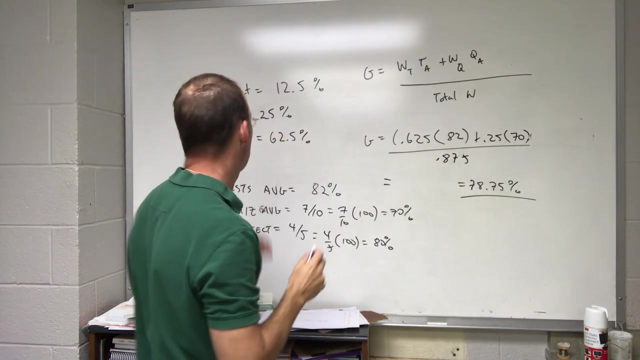 Okay, So my total weight: I'm going to get rid of that. I can get rid of that. Now. my total weight is going to be just these two added together, So that's 87.875.. Is that right? Yeah, .875.. 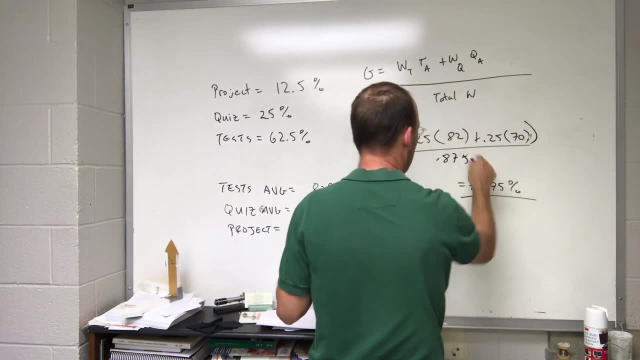 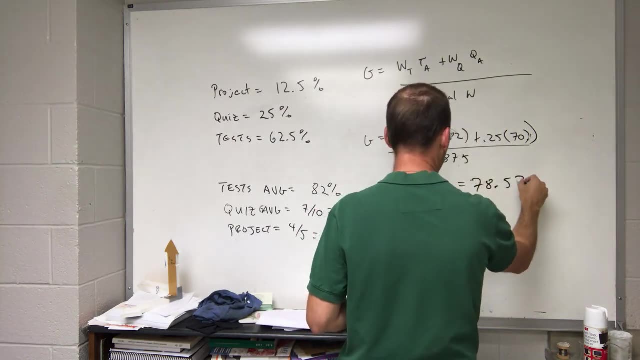 And then if I divide, if I add this up and divide by .875,, I get 78.57.. So it's a little bit lower, because I don't want to get rid of that. I don't want to get rid of that. 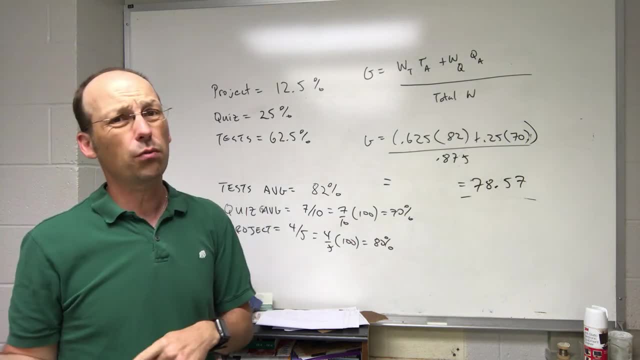 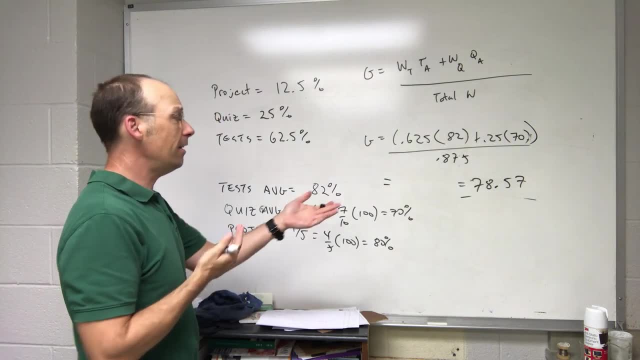 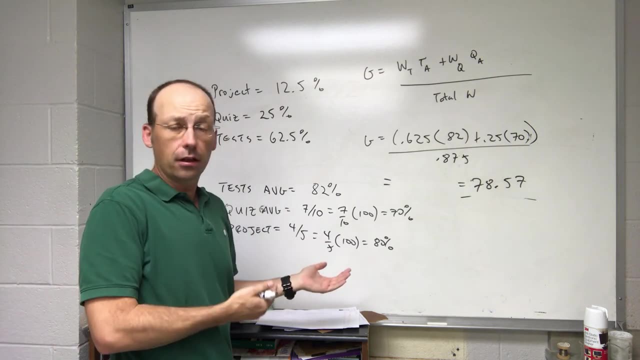 so it really didn't make that big of a difference. And this isn't your grade. I mean, this is the hard thing I have when people say what's my grade? Well, you haven't done the project, so it's really kind of hard to determine what your grade is. 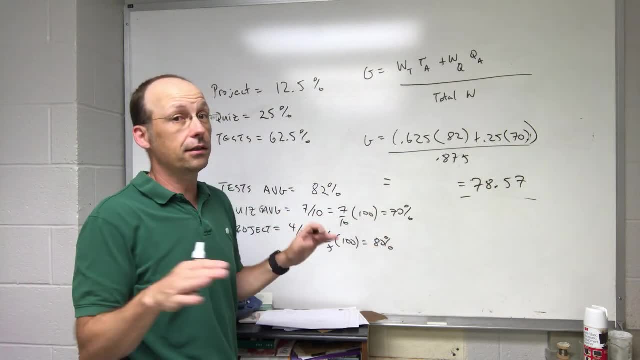 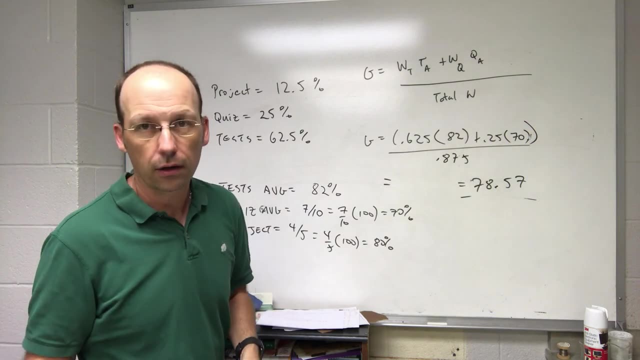 This is your grade. if we said there is no project, Okay, This isn't your grade if you don't do the project, So it could be higher, it could be lower. That's your grade so far. That's what people want. 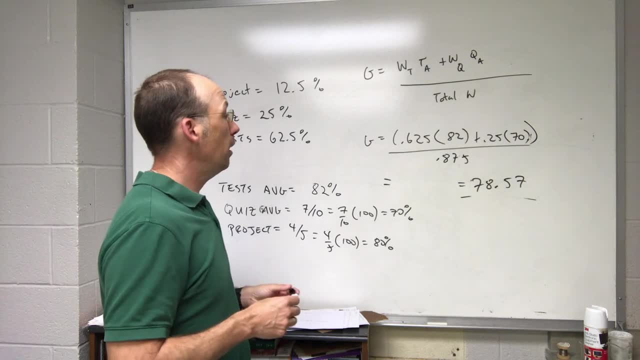 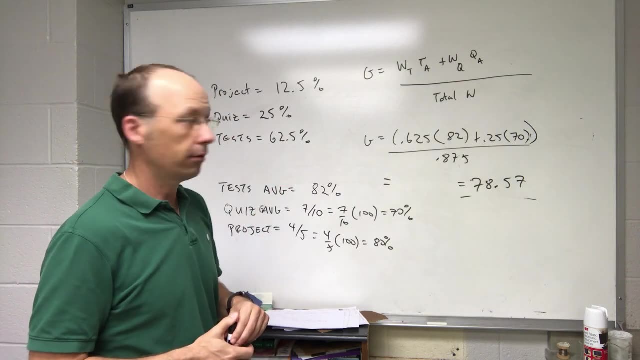 It's the midterm. Let's do one other thing. Let's say: what would I have to get on the project to get a B in the course? Okay, So in that case I'm going to say I know what the grade is going to be.